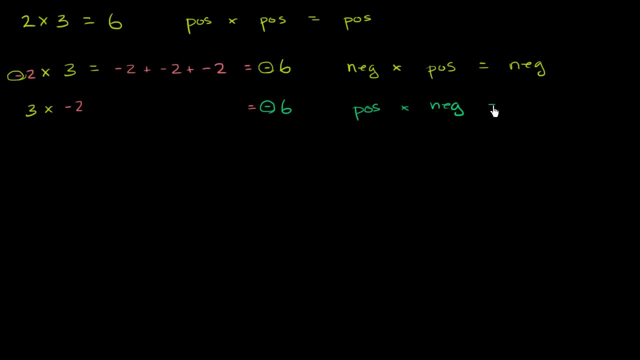 So we could write a positive times. a negative is also going to be a negative, And both of these are just the same thing, with the order in which we're multiplying switched around. But this is one of the two numbers are negative, Exactly one. 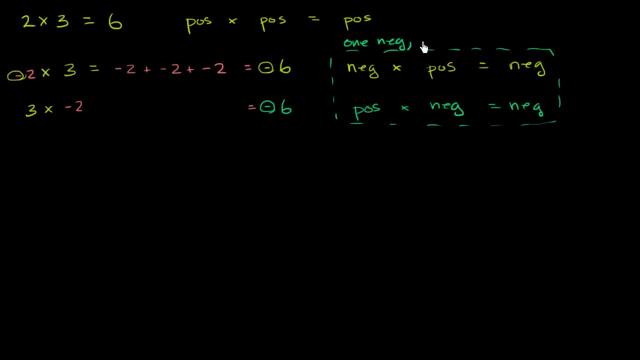 So one negative, one positive number is being multiplied, Then you will get a negative product. Now let's think about this, The third circumstance, when both of the numbers are negative. So if I were to multiply, I'll just switch colors for fun. 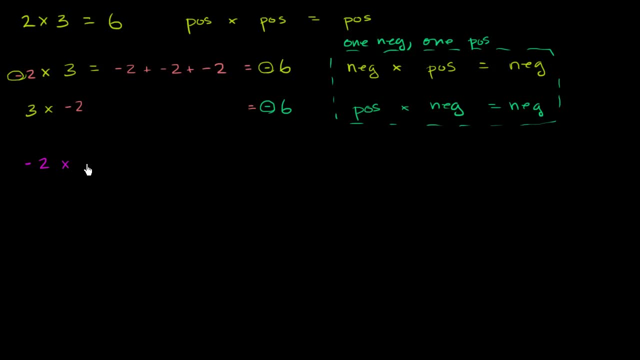 here, if I were to multiply negative 2 times negative 3.. And this might be the least intuitive for you of all. And here I'm just going to introduce you to the rule, And in future videos we'll explore why this is. 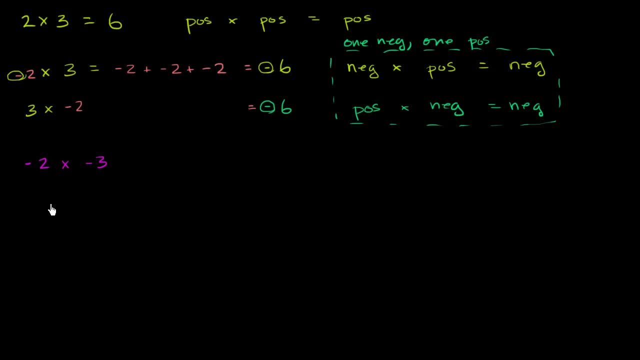 and why this makes mathematics all fit together. But this is going to be. you say: well, 2 times 3 would be 6. And I have a negative times a negative, And one way you can think about it, it is that the negatives cancel out. 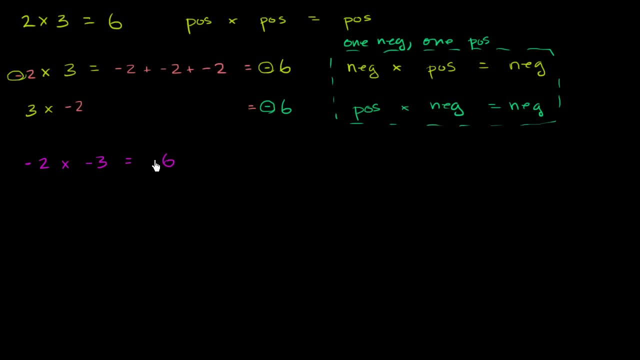 And so you will actually end up with a positive 6.. I actually don't have to write a positive here, but I'll write it here just to re-emphasize This right over: here is a positive 6.. So we have another rule of thumb here. 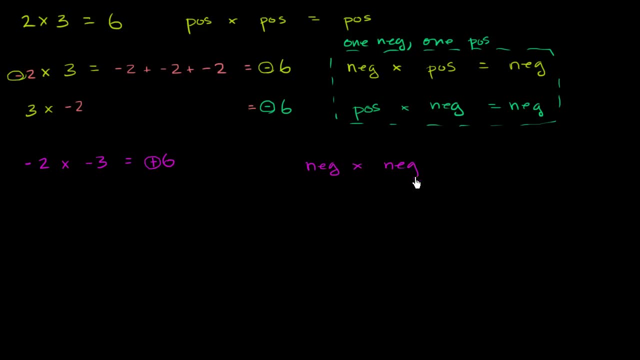 If I have a negative times, a negative, the negatives are going to cancel out And that's going to give me a positive number. Now, with these out of the way, let's just do a bunch of examples And I encourage you to try them out. 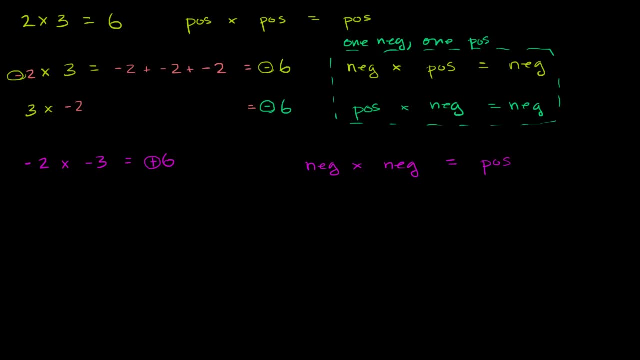 Before I do them, pause the video, try them out and see if you get the same answer. So let's try: negative 1 times negative, 1.. Well, 1 times 1 would be 1. And we have a negative times a negative. 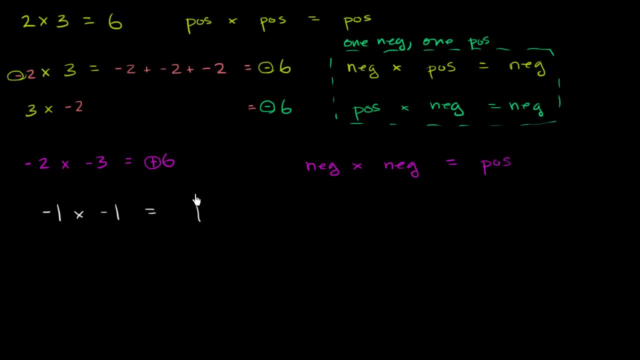 They cancel out Negative times a negative give me a positive, So this is going to be positive 1.. I could just write 1, or I could literally write a plus sign there to emphasize that this is a positive 1.. What happens if I did negative 1 times 0?? 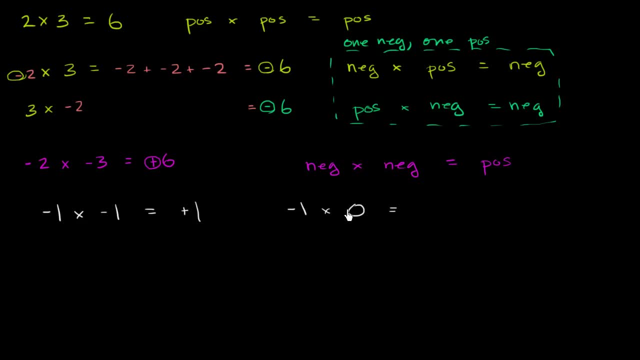 Now this might say: wait, this doesn't really fit into any of these circumstances. 0 is neither positive nor negative. And here you just have to remember anything: times 0 is going to be 0.. So negative 1 times 0 is going to be 0..